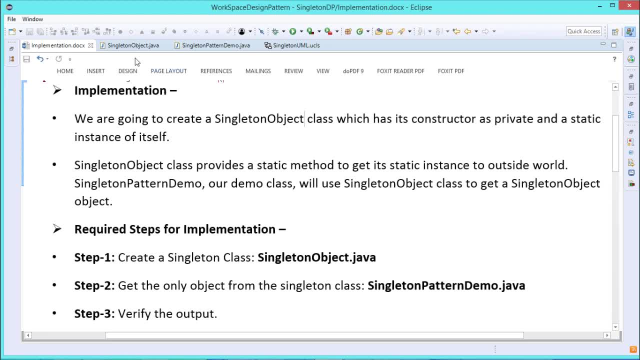 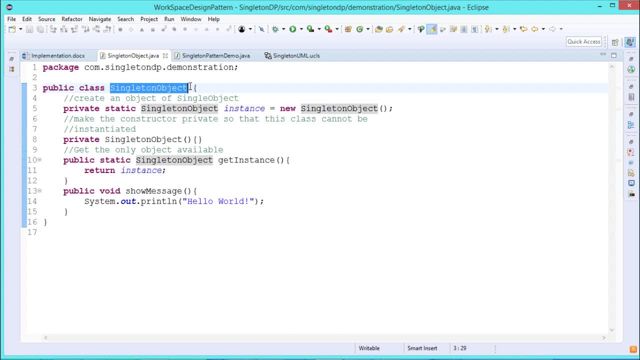 So we will be going for the output. So now let us come to the coding part for the better understanding. So here we are having one class that is a singleton object, The name of the class is singleton object and it is having its own instance, static singleton. 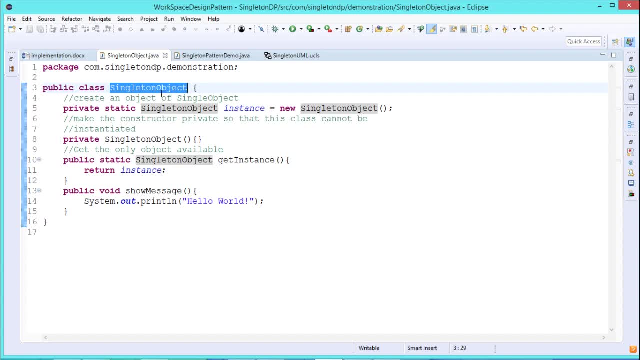 object instance is equal to new singleton object, So it is having its own instance variable and the name of this variable is this instance. So there is a message we are having. So there is a member variable and this is our singleton object. So we are going. 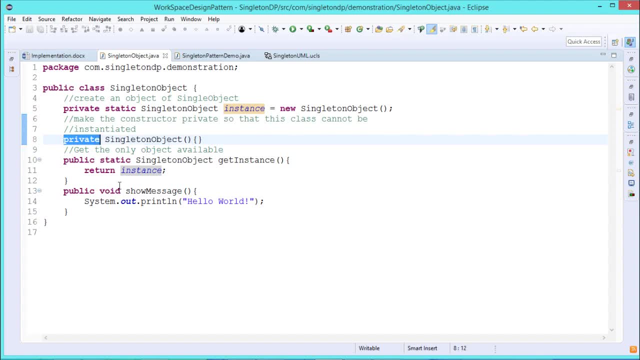 to use singleton object. we are going to mix up the same thing, So this is the form of a singleton object, So we will be using singleton object. The name of the singleton object is the constructor which is defined under the private scope. that is very important. 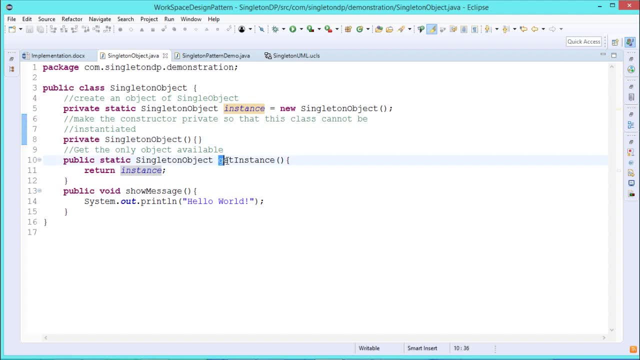 which is defined under the private scope. So that is, make the constructor private so that this class cannot be instantiated using this constructor and to get the only object against this class- And that is the basic theme behind this singleton design pattern method- this one and singleton object will be returned, and it is returning this instance. so 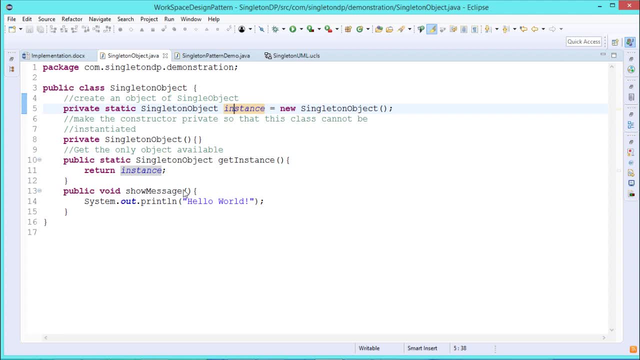 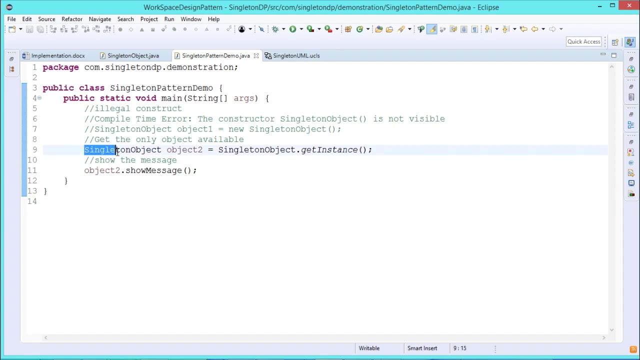 it is returning this instance. here we are having one method. there is a show message that is the systemout of println. hello world. so this is my singleton object class. so now let us come to this singleton pattern demo. so here you see, we have defined this particular singleton object object. 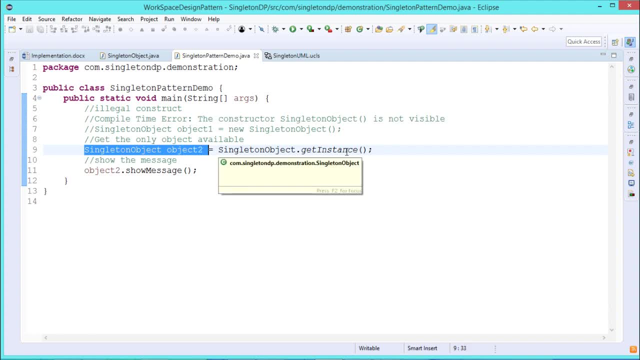 is equal to is equal to singleton object dot, get instance. you know that, get instance, is is a method which was under the public section, under the singleton object class, and which was of the type static. so that's why object name dot, get instance, this method can easily be called, so for. 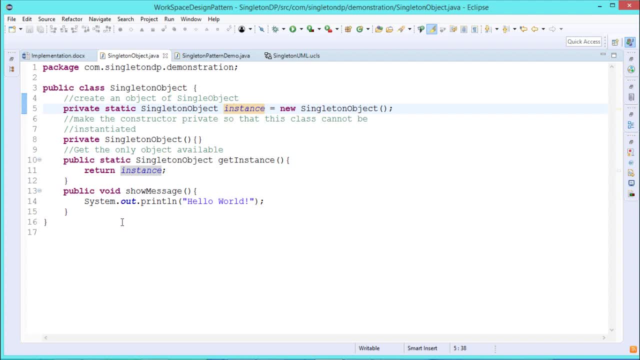 the later visualization. i'm just putting the code, singleton object, in front of you. you can find that it is under the public scope, this particular method get instance, and it is of the type static. so so as a result of that singleton object dot get instance method, we can also easily call: 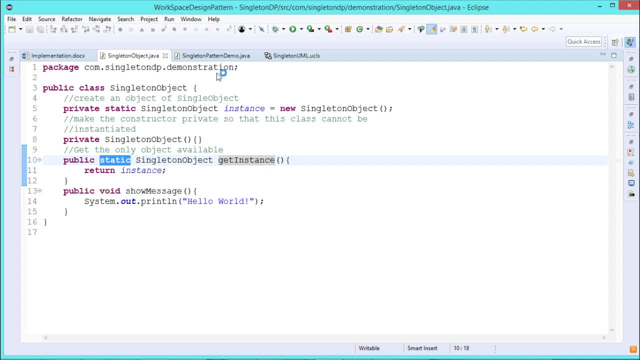 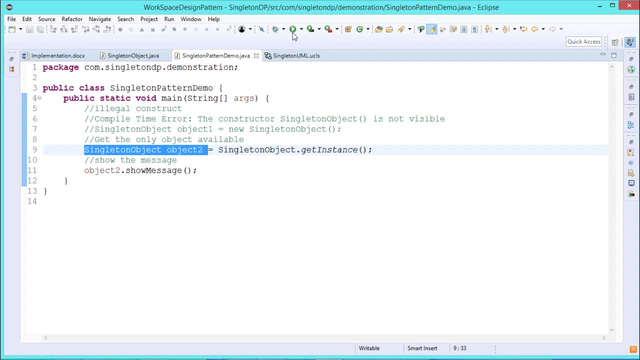 and it returns singleton object as the output argument. so that has been put in object two and later object two dot show message will print the hello world message. so now we are getting this hello world here. so now see, if we want to define this singleton object object, let it be object one.